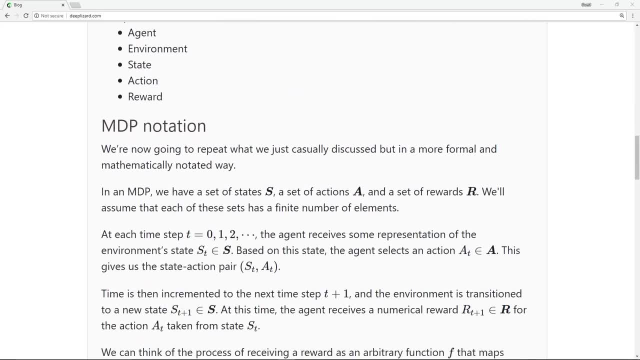 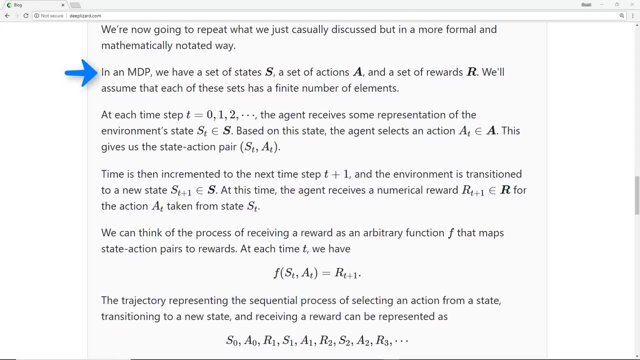 This will make things easier for us going forward. So we're now going to repeat what we just casually discussed, but in a more formal and mathematically notated way. In an MDP, we have a set of states- big S, a set of actions, big A and a set of rewards. 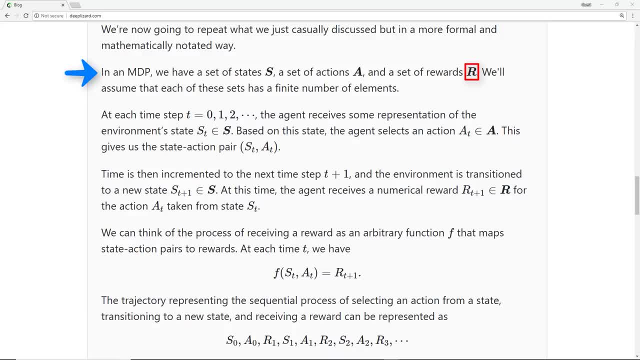 big R. We'll assume that each of these sets has a finite number of elements. At each time, step t, the agent receives some representation of the environment's state S sub t. Based on this state, the agent selects an action, A sub t and together this state. 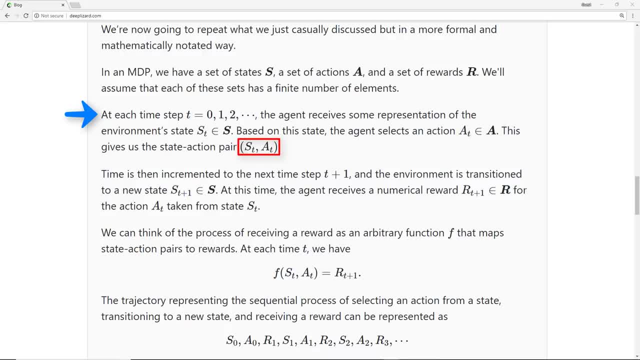 and this action gives us the state-action pair S, t comma A. t Time is then incremented to the next time step t plus 1, and the environment is transitioned into a new state. At this time the agent receives a numerical reward- R t plus 1, from the action taken from. 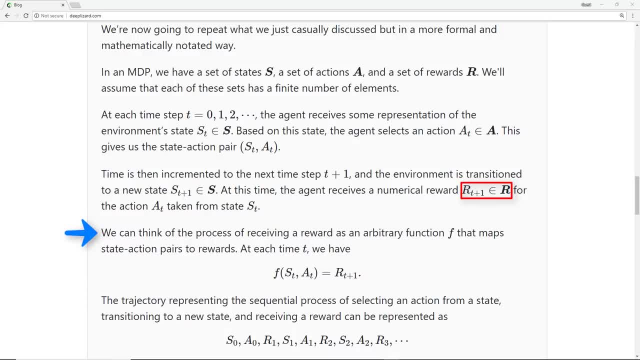 the previous state. So generally we can kind of think of this process of receiving a reward as an arbitrary function that maps state-action pairs to rewards. The trajectory representing the sequential process of selecting an action from a state and then transitioning to a new state and receiving a reward can be represented like: 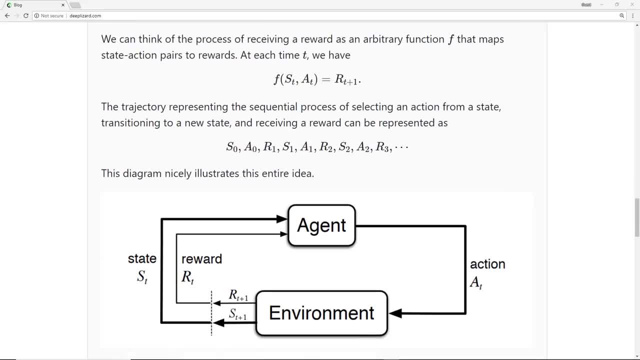 this. This diagram nicely illustrates this entire idea. Let's break this diagram down into steps. Step 1. At time t, the environment is in state S, t. Step 2. The agent observes the current state and selects action A, t. 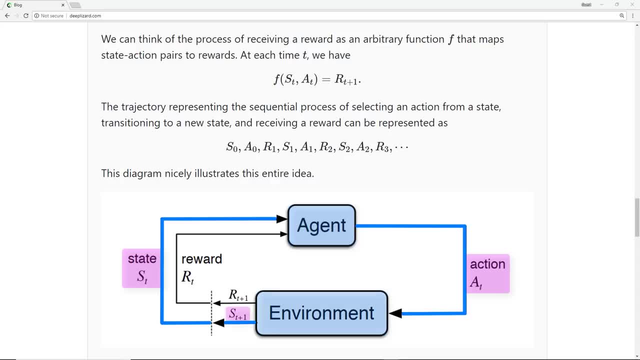 Step 3. The environment transitions to state S t plus 1 and grants the agent reward R t plus 1.. This process then starts over for the next step, Step 4.. At time t, the environment is in state S t plus 1 and grants the agent reward R t plus. 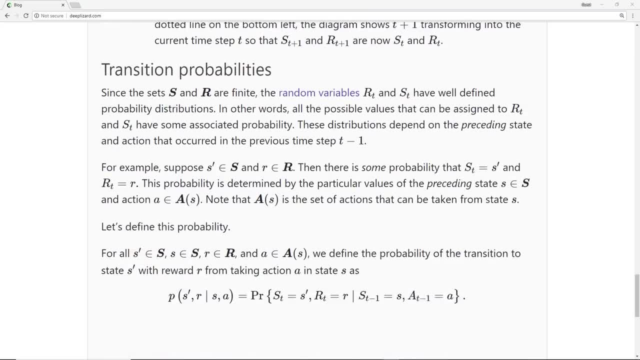 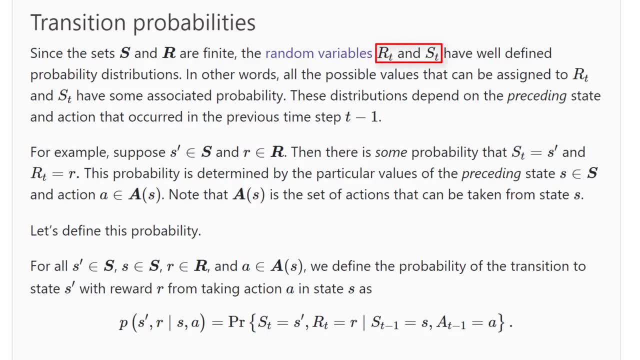 1.. This process then starts over for the next time, step t plus 1.. Now, since the set of states and the set of rewards are finite, the random variables R, t and S, t that represent the reward and the state at time, t, have well-defined probability. 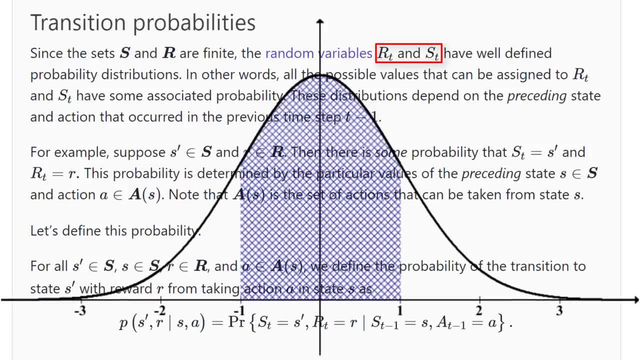 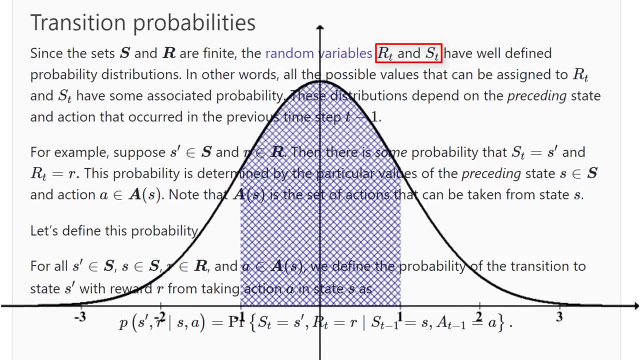 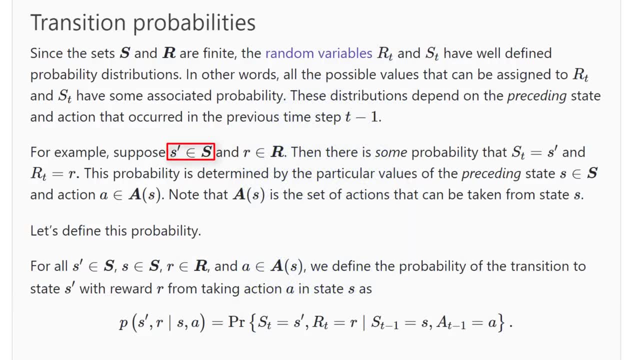 distributions, In other words all the possible values that can be assigned to R, t and S? t, have some associated probability. These distributions depend on the preceding state and action that occurred in the previous time, step t minus 1.. So, for example, suppose S' is a state within the set of all states and R is a reward within 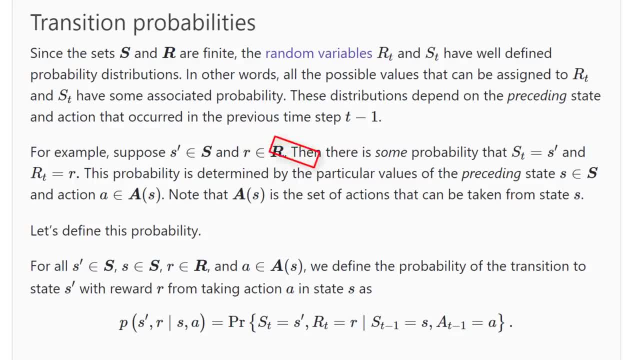 the set of all rewards. Then there is some probability that the state at time t will be S' and that the reward at time t will be R. This probability is determined by the particular values of the preceding state and preceding action. We have a bit more formal details regarding transition probabilities on this slide, but 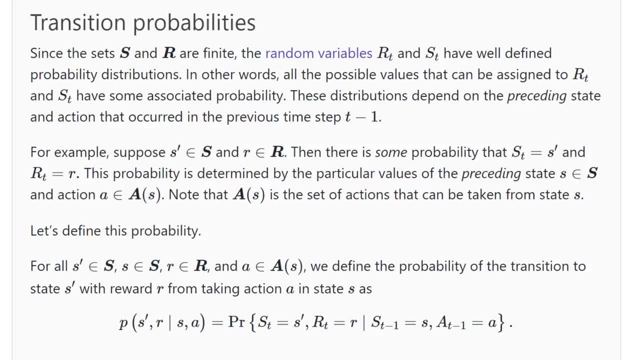 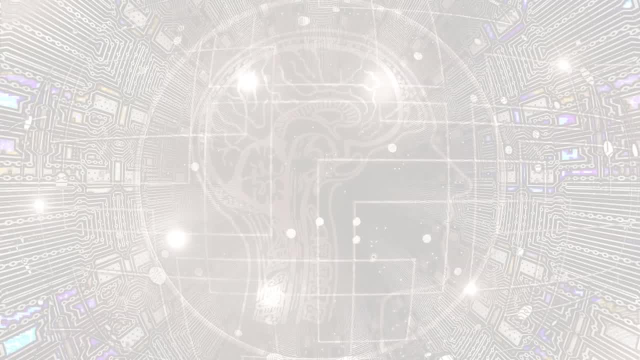 we'll get to that later. It's on the corresponding blog for this video on deeplizardcom, so be sure to check that out. Alright, we now have a formal way to model sequential decision making. How do you feel about Markov decision processes so far? 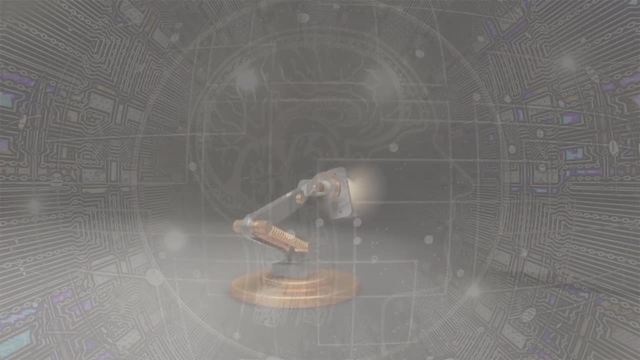 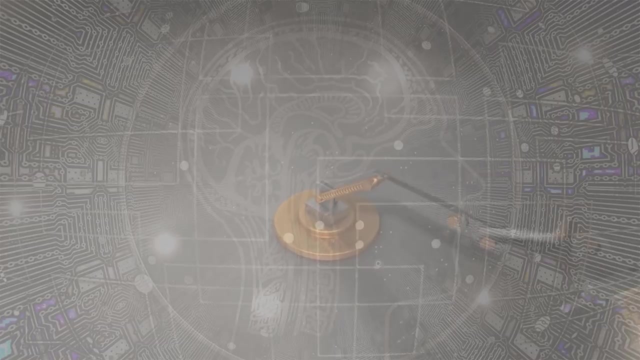 Some of this may take a bit of time to sink in, but if you can understand the relationship between the agent and the environment and how they interact with each other over time, then you're off to a great start. It's a good idea to utilize the blog for this video to get more familiar with the mathematical 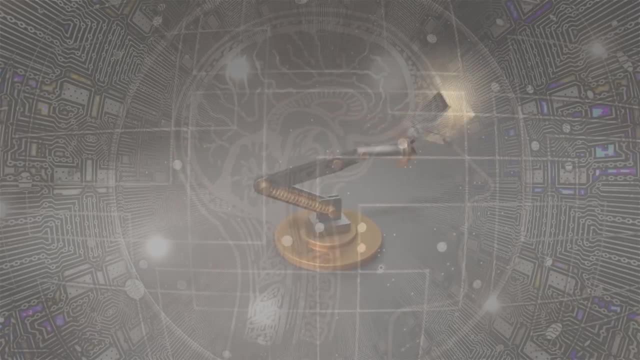 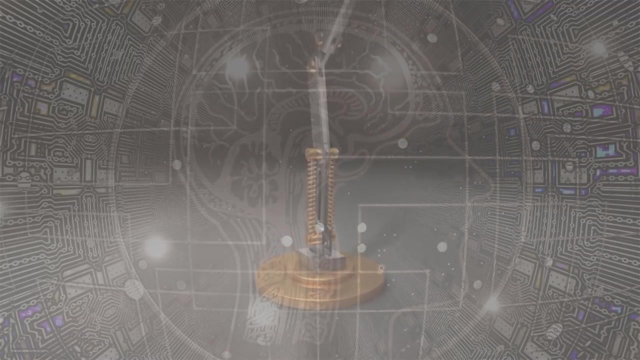 notation. We'll be seeing it a lot in future videos And, while you're at it, check out the Deep Lizard Hivemind for exclusive perks and rewards. Like we discussed earlier, MDPs are the bedrock for reinforcement learning, so make sure to. 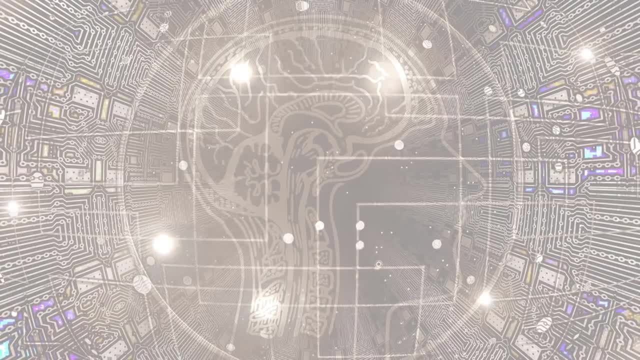 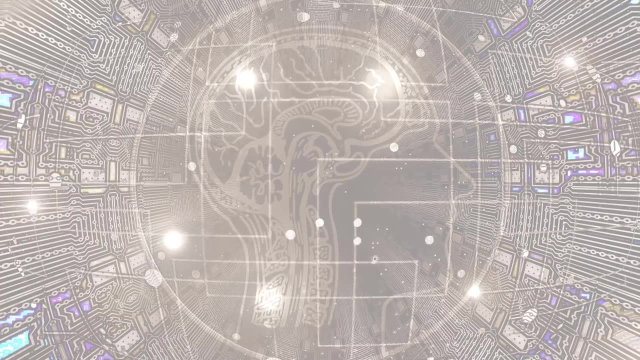 get comfortable with what we covered here, and next time we'll build on the concept of cumulative rewards that we introduced earlier. Thanks for contributing to Collective Intelligence and I'll see you in the next one. Do they have detection, the humans? That is the question. 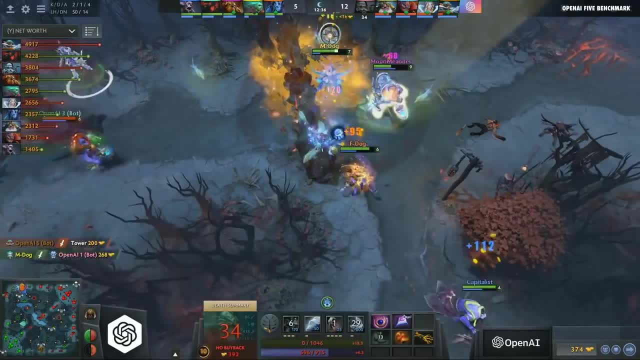 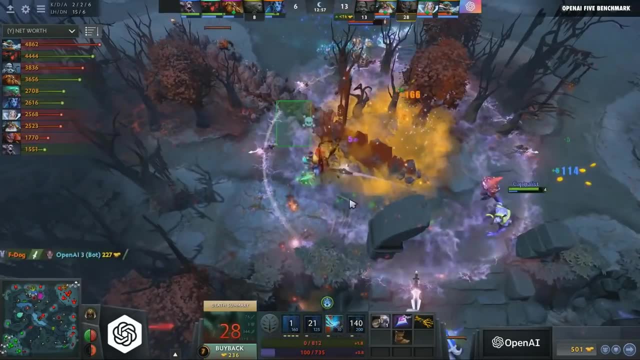 They're learning. It's not enough to know. It's not enough to know. It's not enough to save it, though. They find the kill Quick finger, though, as the counterplay comes in, from OpenAI, In fact, jumping back in with the silence, he's got the tricks of the trade and they'll